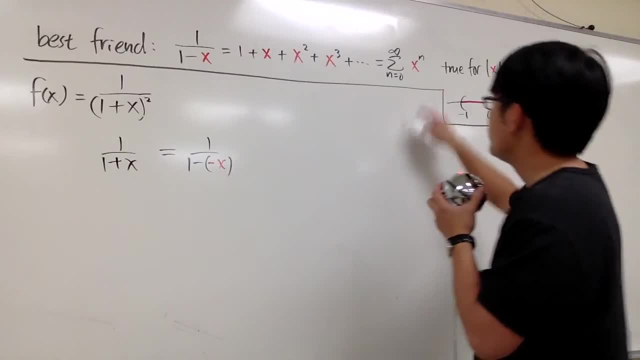 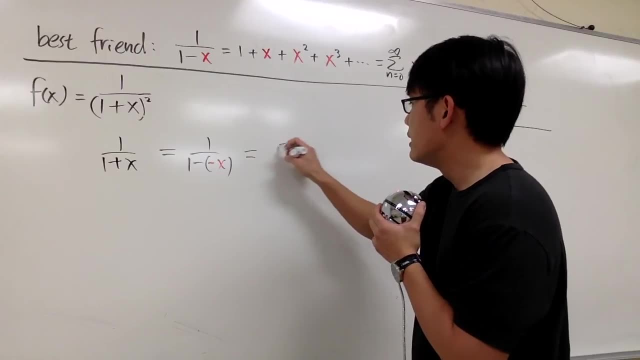 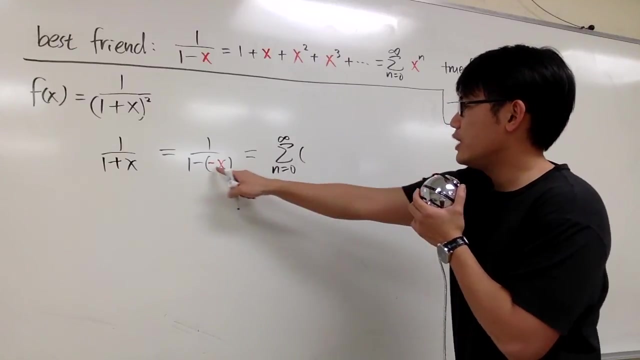 So that we have the right to plug in negative x into this x, And we'll just work with the sigma notation right here. okay, This is the same as sigma when n goes from 0 to infinity Negative 1, because here we have negative x. 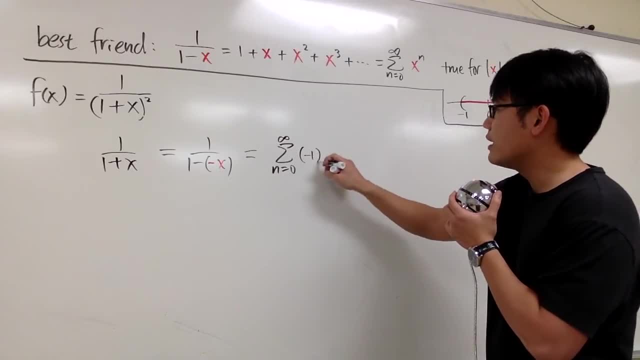 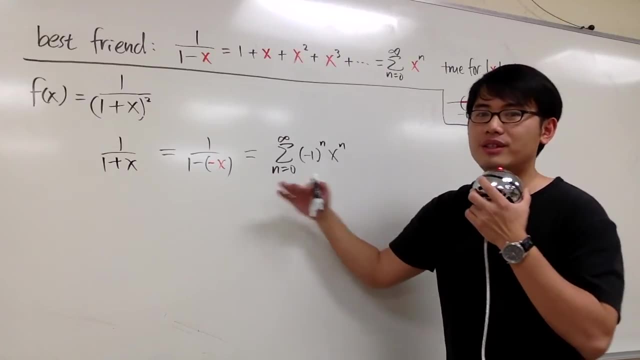 negative 1 times x. So we can write this down as negative 1 to the nth power first and then times x to the nth power. okay, And then in fact I did another video in more detail, explanation of this one, so you can check that out. 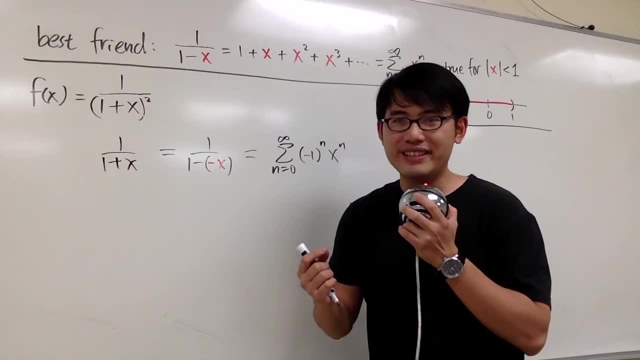 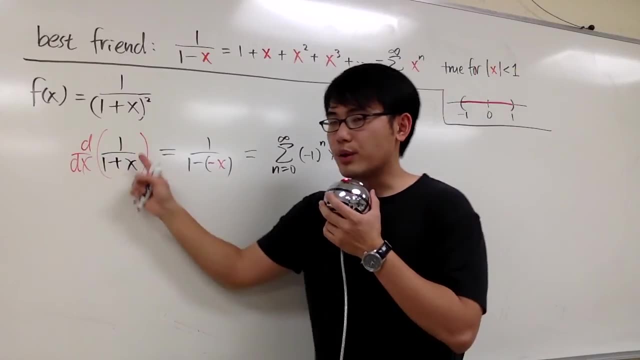 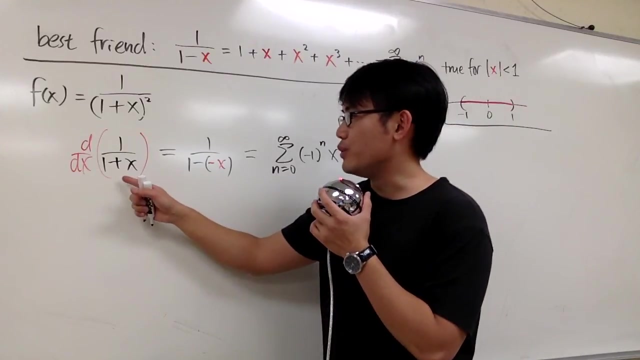 But then we need to use this first and then differentiate. Let's show you how to differentiate: 1 over 1 plus x. This is the quotient. and then the quotient rule says we have to square the denominator right. You see, that's a hint on why we should use differentiation. 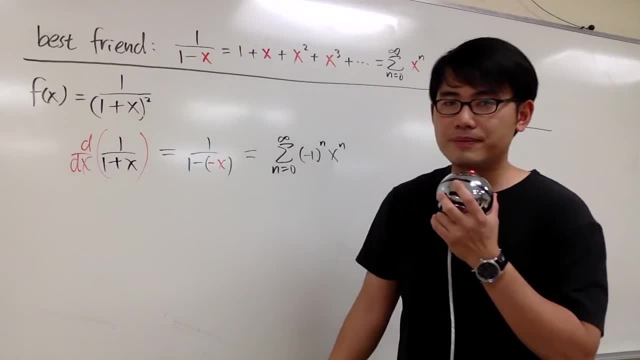 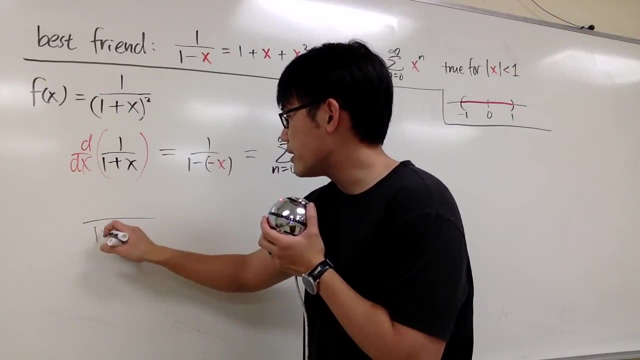 because this function is something square on the denominator. Anyways, I'll show you how to differentiate this with the quotient rule. This right here we first look at the denominator 1 plus x, put that in the parentheses and then raise that to a second power. 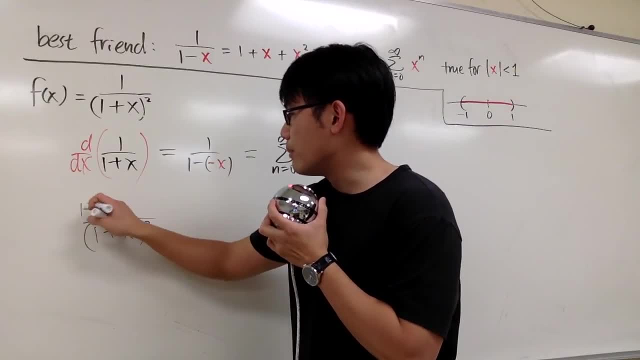 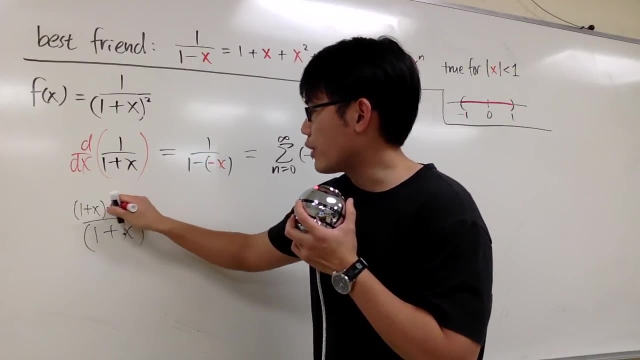 And the quotient rule says we will put down the bottom function, which is 1 plus x times the derivative of the top derivative of 1, 0. So we have the 0 right here, And then we subtract the top function, which is 1,. 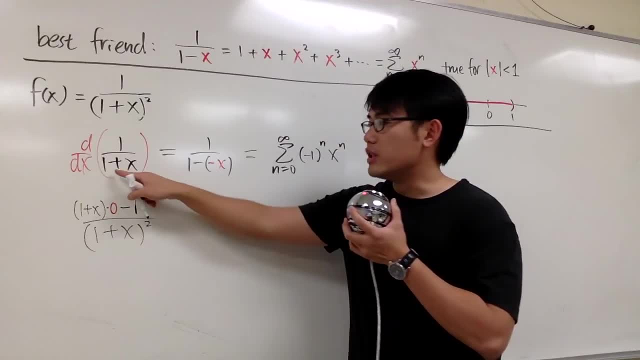 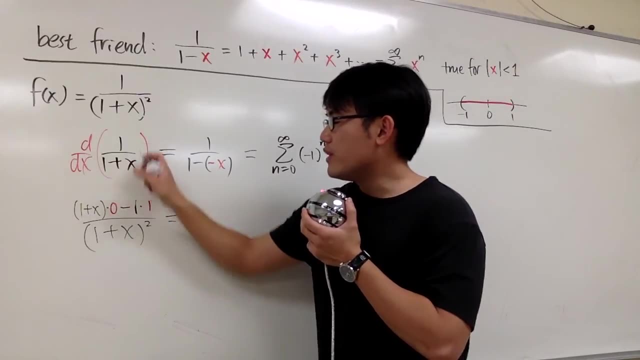 times the derivative of the bottom function Derivative of 1 is 0,. derivative of positive x is 1, so multiply by 1.. So in another word, the derivative of this is going to be: well, this is 0,. negative 1 times 1 is negative 1,. 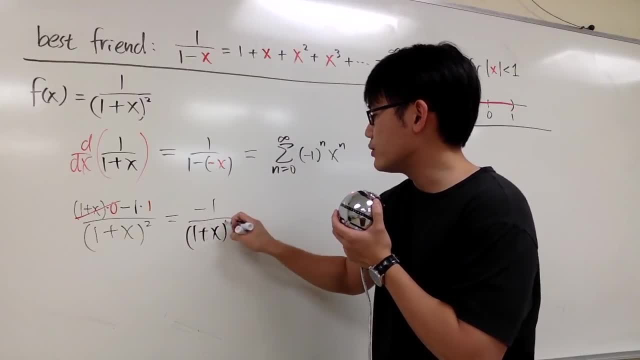 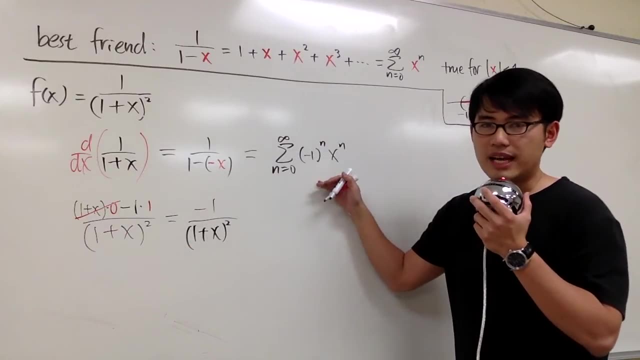 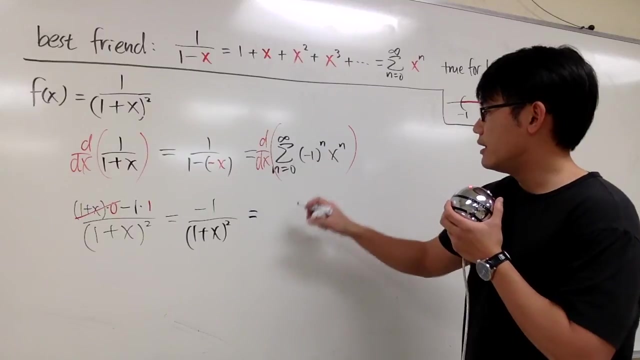 over this 1 plus x and then raise to a second power. So we differentiate this inside, we get that, And we also differentiate The right-hand side, the dx. So this is going to be the same as- let me just put down sigma- when n starts with some number raised to the infinity bar. 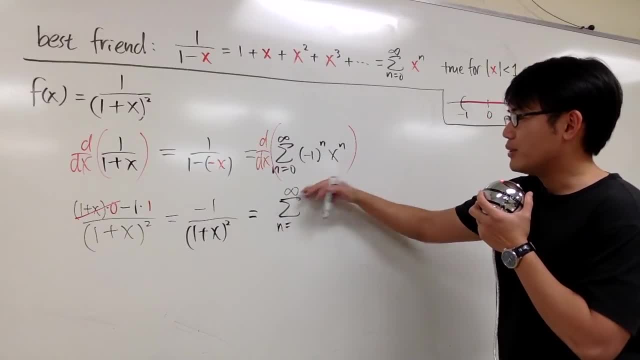 right, well, not raised to infinity. n starts with some number up to infinity And to differentiate this, this is just like a number, so we can just put down negative 1 to the nth power. This is the function part x to the nth power. 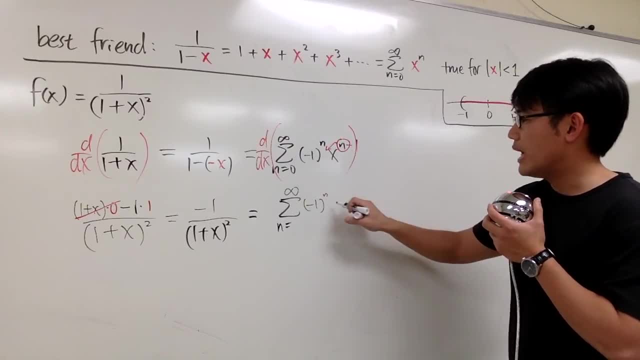 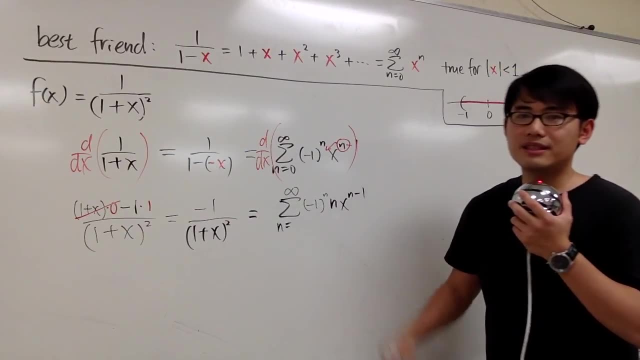 We bring the power to the front and then minus 1, so we have n times x to the nth, minus 1 power. This is the same as that. And one more thing is that, well, what should be our starting value for n? 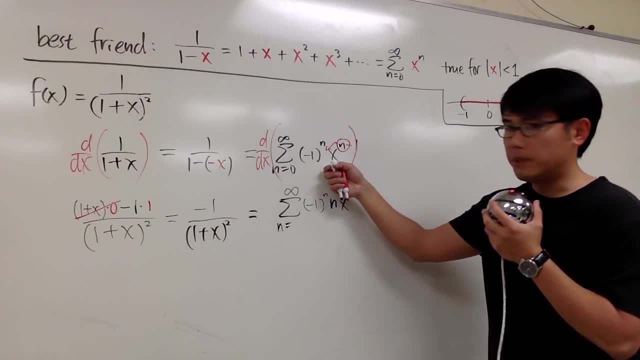 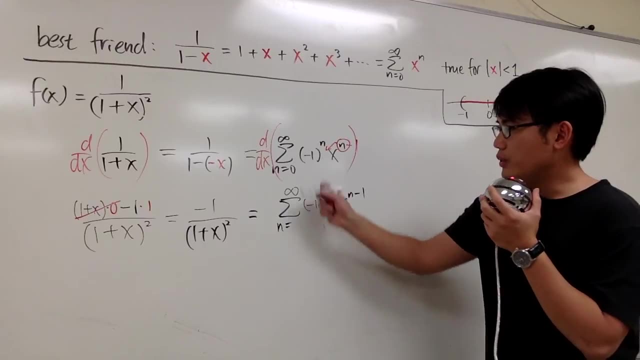 This is one thing that we can do real quick. Whenever we differentiate a power series, we'll lose one term, most likely, And the key is, you can first just maintain the same term. for example, n is equal to 0.. 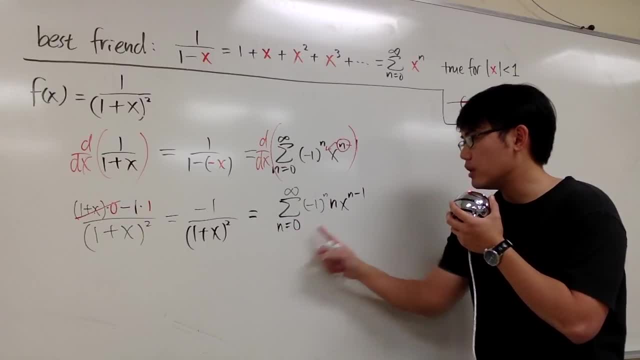 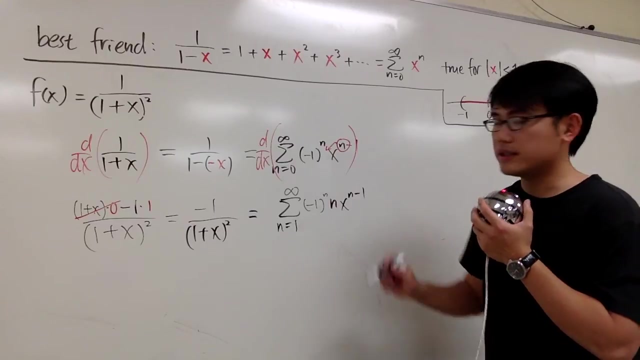 But then you see that the moment when you plug in n is equal to 0 into this equation, into this formula, here the first term, you'll produce 0, because you have this n And we like to avoid redundancy, So we will start with: n is equal to 1 instead. 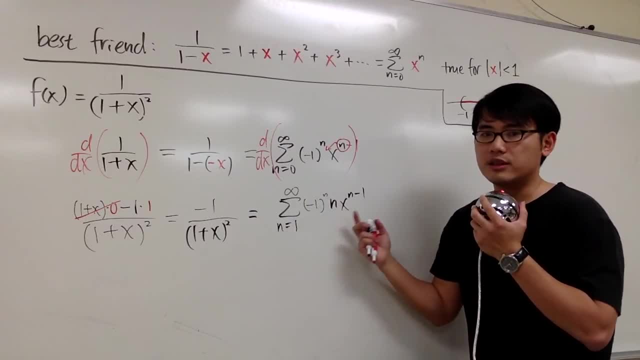 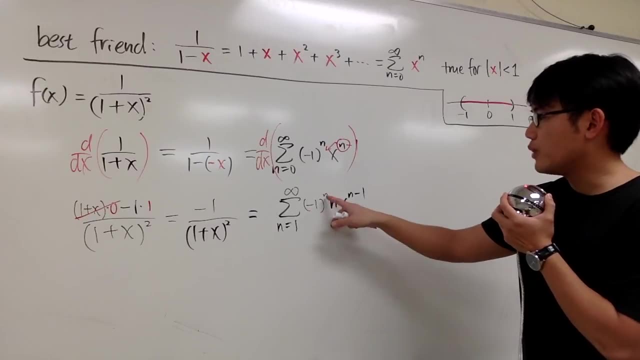 When n is equal to 1, we will produce our first non-zero term And you will. you know, just plug in 1 to all the n you'll produce. I think the first term is going to be negative: 1 to the n. 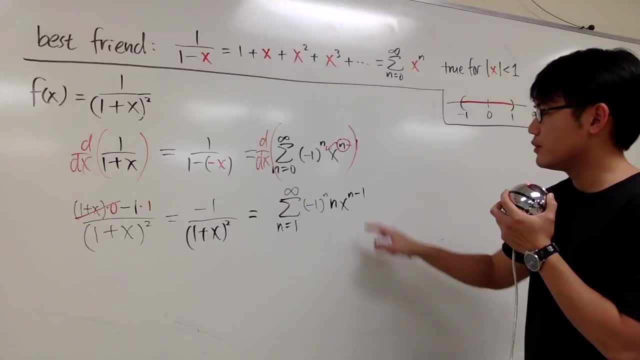 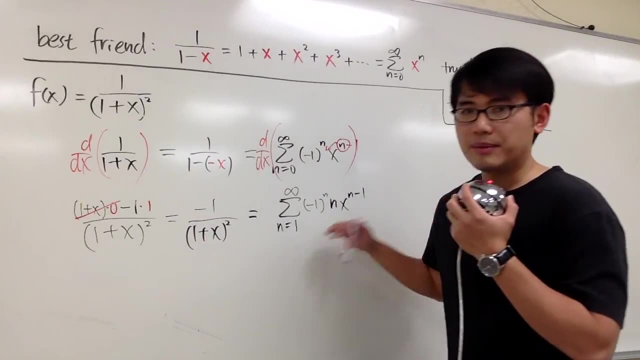 Which is 1 times 1 times x to the 0 power, 1 minus 1.. So you have negative 1 for the first term. Anyways, this is the same as that, But then our original function is positive 1 on top. here we have negative 1.. 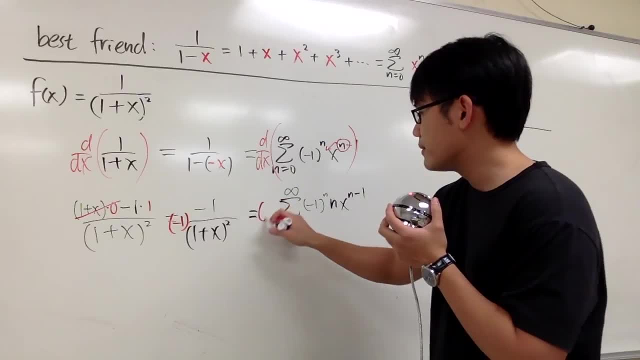 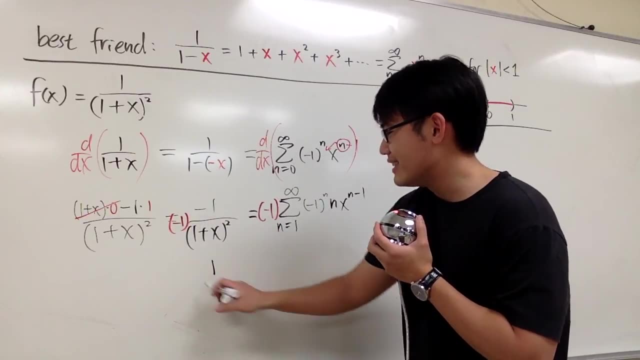 Well, not that bad, because we can multiply both sides by negative 1.. Let's do that: Negative 1 times 1, I mean negative 1 times negative 1, we have positive 1 on the top over 1 plus. 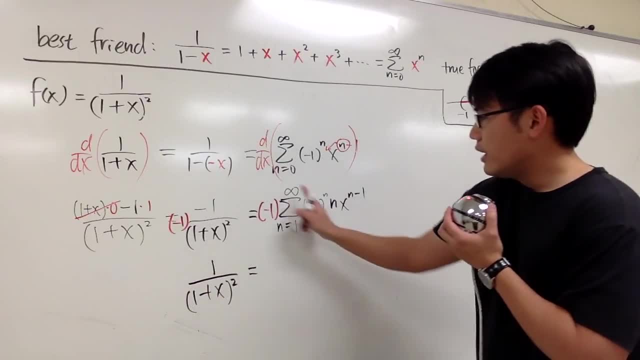 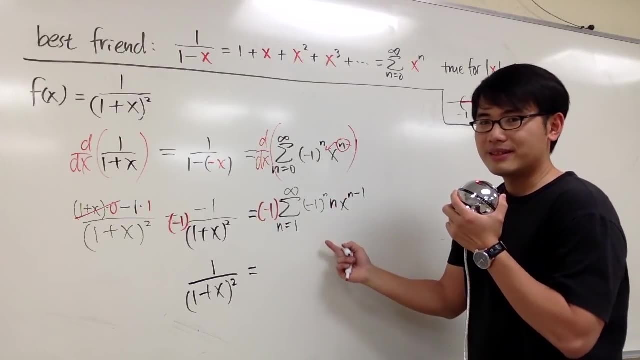 x raised to the second power. And then for this, right here, I will just multiply out the negative 1 into this. Multiply the inside, okay, not multiply the out. multiply this and that I will keep the same single notation. n goes from 1 to infinity. 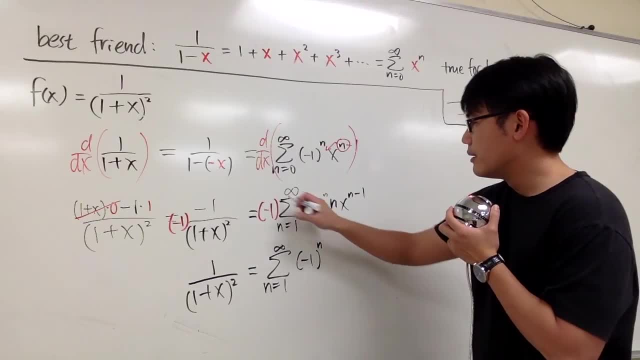 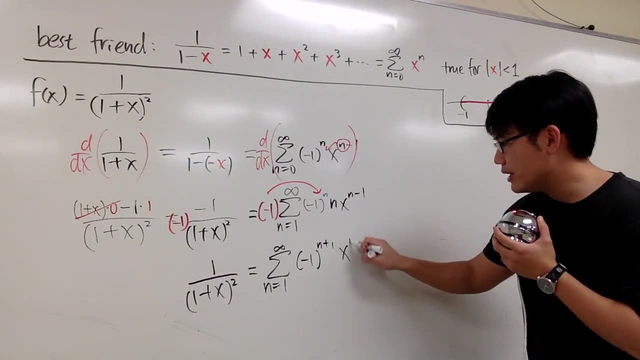 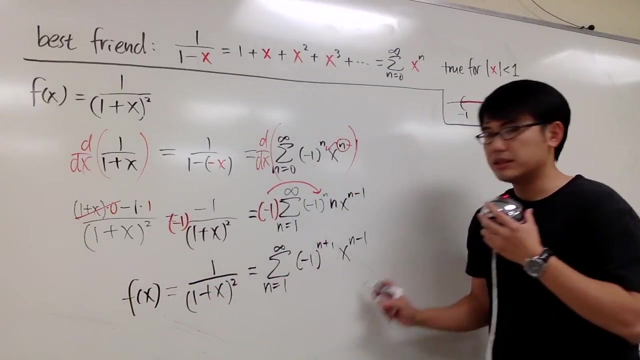 This will be negative: 1 to the n power plus 1, because I multiplied this with that, And then we have the x to the n minus 1 power And that's pretty much it. f of x, which is this function. which is that, that's the power series expansion. 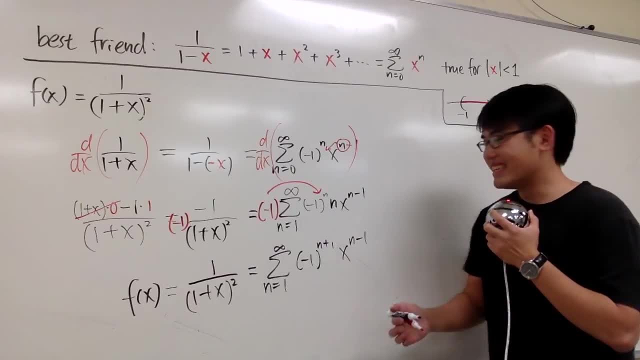 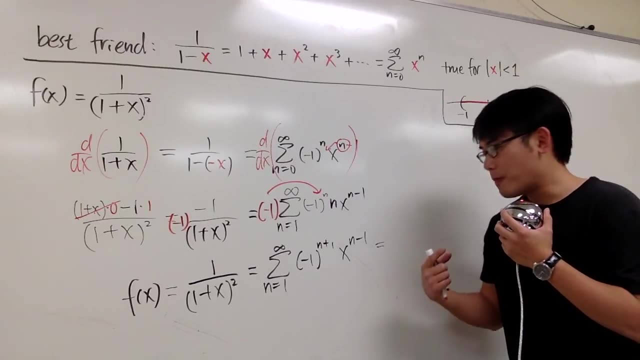 But in the the answer in the back of the book, this is what they do: They want to have x to the n power instead of x to the n minus 1 power. So what they do is they look at this formula here. 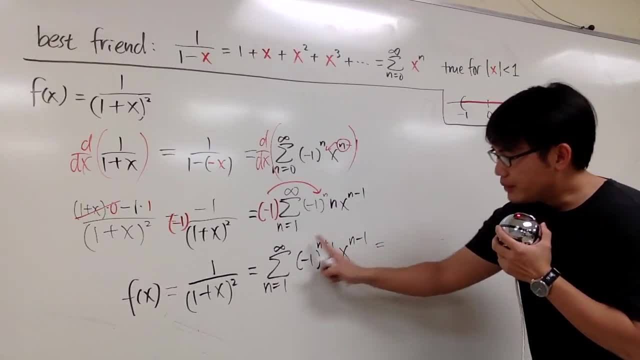 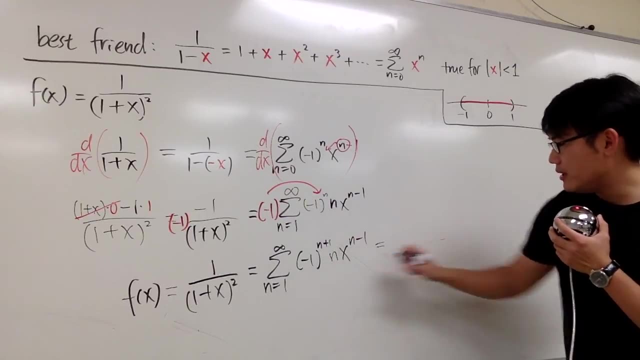 Oh, by the way, I forgot earlier, They look at this formula here. They just add 1 into all the n. So let me show you This is going to be negative 1 to the n, plus 1, and then plus 1.. 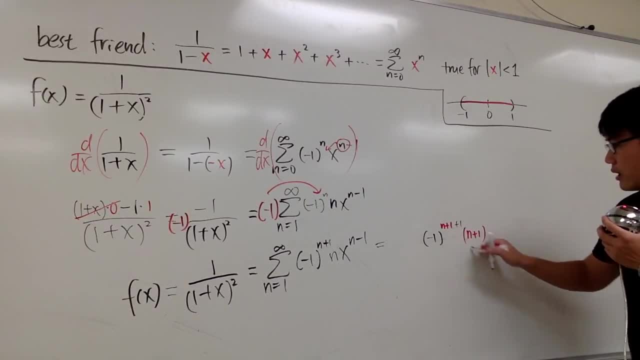 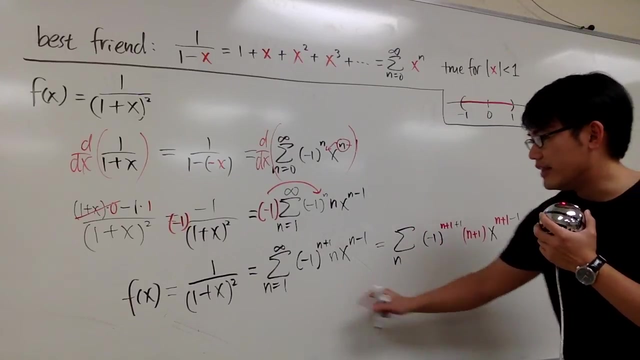 And then this n becomes n plus 1.. And then this n becomes n plus 1.. But then we still have the minus 1 there. So they add 1 to all this n, But then, to compromise that, they subtract 1 from the starting value. 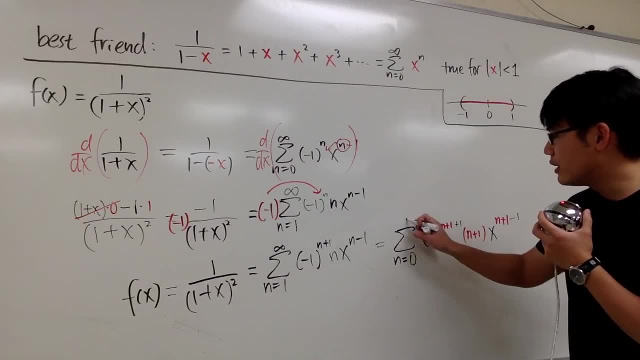 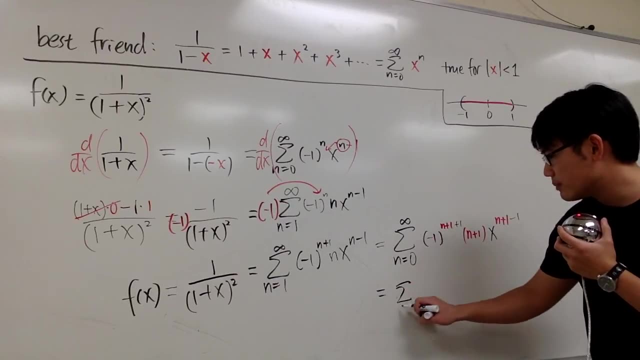 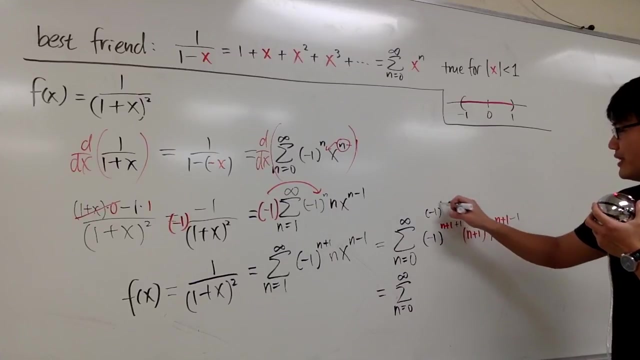 So instead of 1, it becomes n is 0 up to infinity. At the end we can simplify this a little bit. This is going to be sigma when n goes from 0 to infinity, And then this is negative 1 to the n plus 2 power. 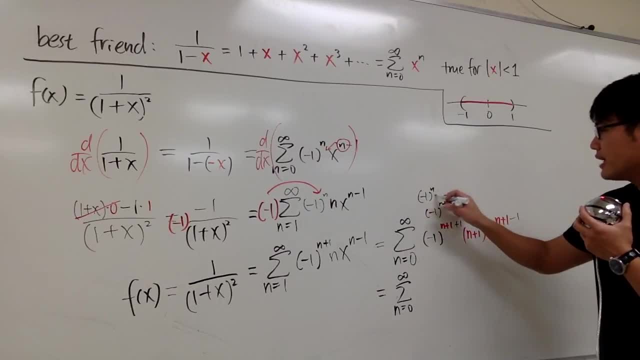 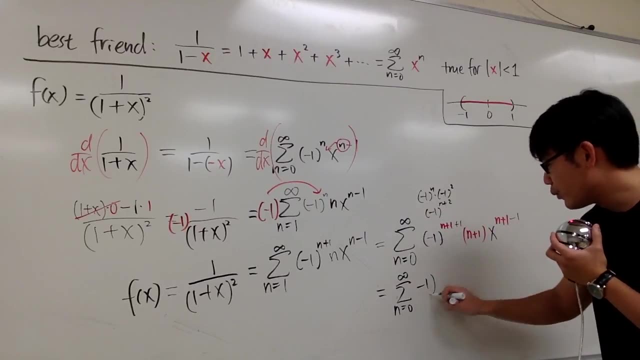 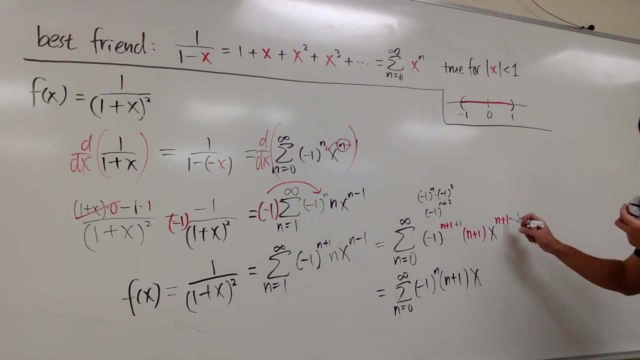 And if you break this apart, this is the same as negative 1 to the n times negative 1 to the second. This is just 1.. So we just met, We just care about Negative 1 to the nth power times: n plus 1 times x to the n plus 1 minus 1, which is n. 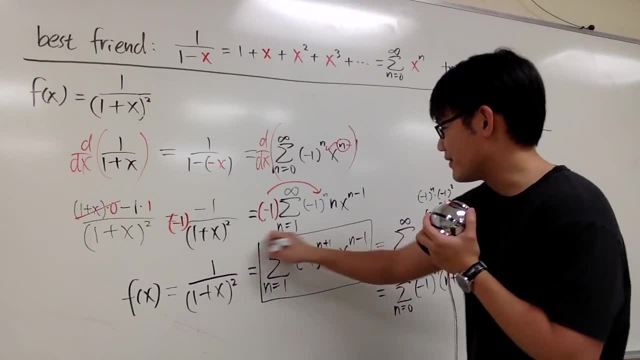 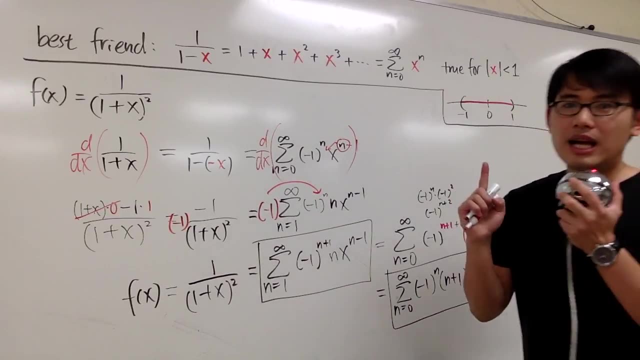 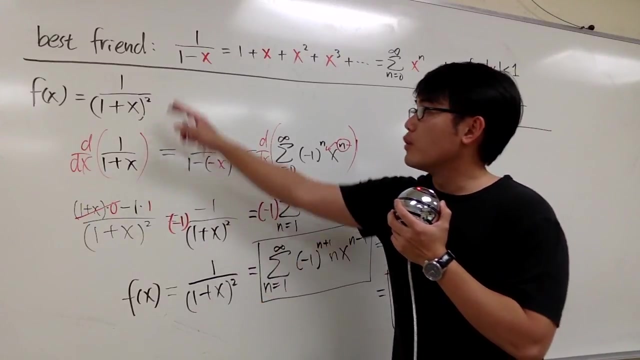 So well, this is just as fine, actually, But then this is the answer in the back of the book, But both of them are equivalent to that. However, this is an important thing that I have to tell you Whenever you use differentiation with our best friend, either version. 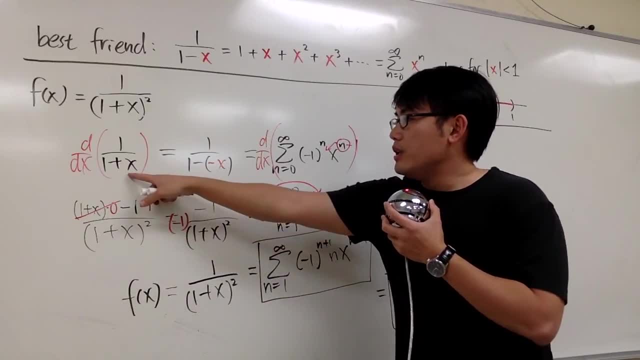 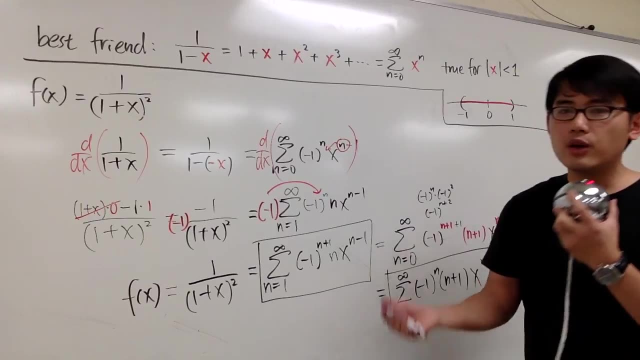 because this is not really our best friend. we differentiate this and then we come up with the power series for this function. If that's the case, whenever we differentiate or integrate with a version with our best friend, the radius of convergence stays the same. 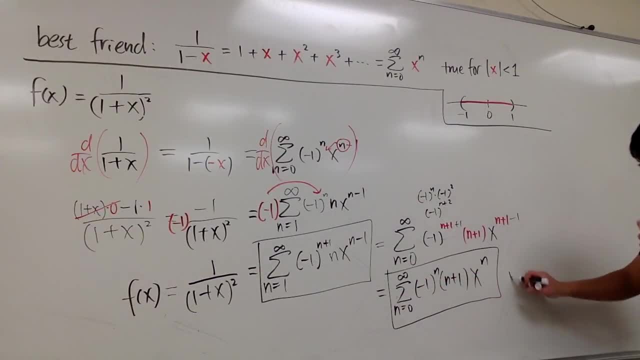 So in this case, we know this is the form, but then we should also include that the radius of convergence is r is equal to 1, because earlier r was equal to 1 for our best friend, And then r was equal to 1 with this as well. 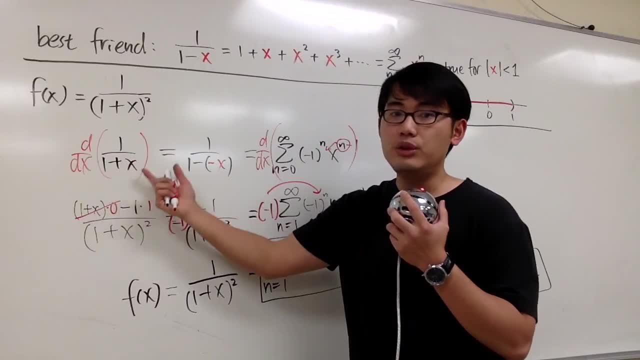 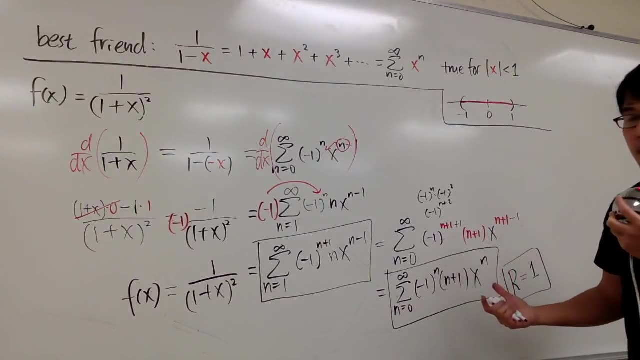 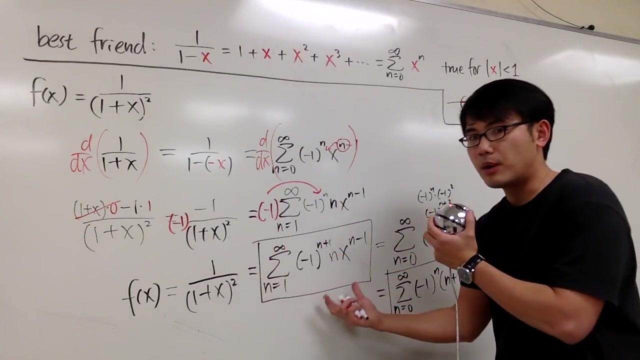 You have to worry when we have, let's say, 1 over 1 plus 3x, things like that, or 1 over 1 minus 4x squared things like that, Then the radius of convergence may change, And whenever we differentiate or integrate the function and then get the power series.